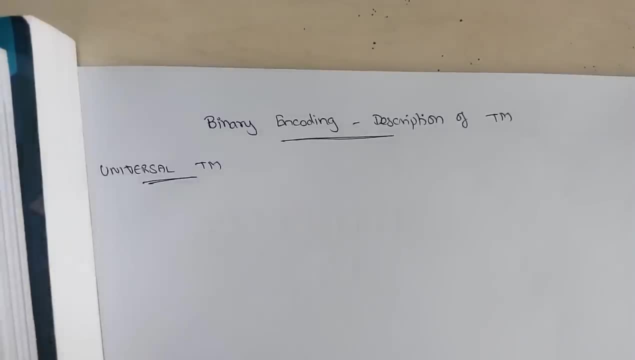 Till now we saw what a Turing machine is Like. we have a Turing machine that do some process. We give a program or for some logic, it works out. Now we will see what is a universal Turing machine. Universal Turing machine is one that runs the description of other Turing machine. 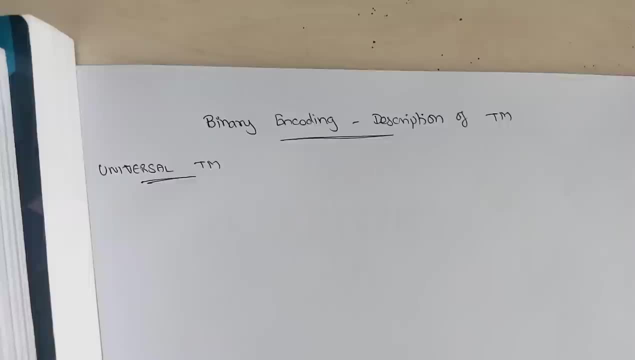 So this universal Turing machine is capable of simulating other Turing machine. So when you give a Turing machine description with an input, if the machine goes to accepting state, then your universal Turing machine will also accepts it. So this is a universal one which has a capability of simulating other Turing machines inside it. 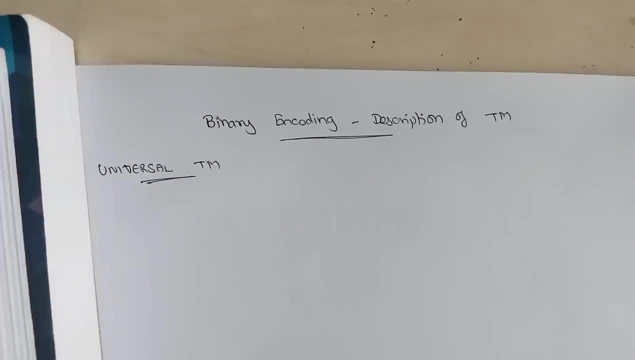 And, like the input given for the universal Turing machine, is a binary, encoded format of a Turing machine. I will just give you a simple example of how to encode a Turing machine binary. So this is a description for a Turing machine. Specifies a final set of state, final set of input symbol that can be represented in a Ts Del is a transition function, Q0 is a starting state and B is a blank representation and F is the final state. 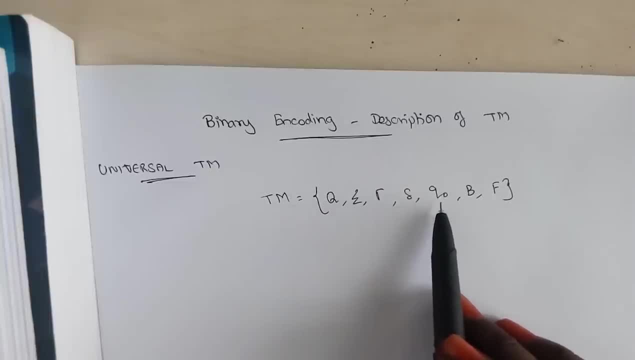 So this is the description for a Turing machine. Now we are going to describe a Turing machine, to consider an example of how to encode that Turing machine. This was a sample of a Turing machine currently in the UK and I will give you an example in binary format. 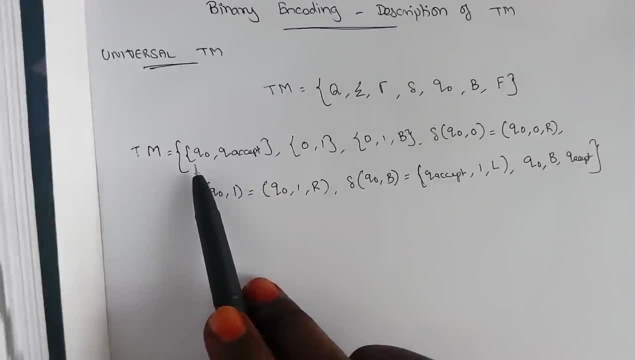 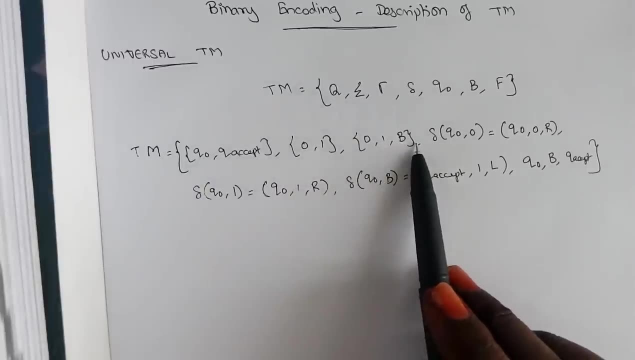 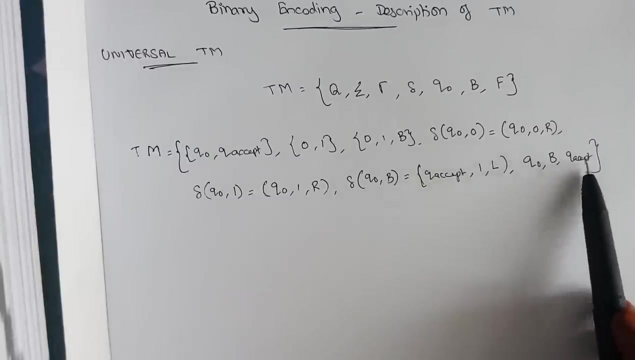 So let us consider an example like this. Here, Q0 and Qexcept are the set of states and the input symbols are 01 and the elements that are written in the tape is 01- blank, and the transitions are given like this: Q0 is a starting state, B is a representation that is used for a blank representation, and 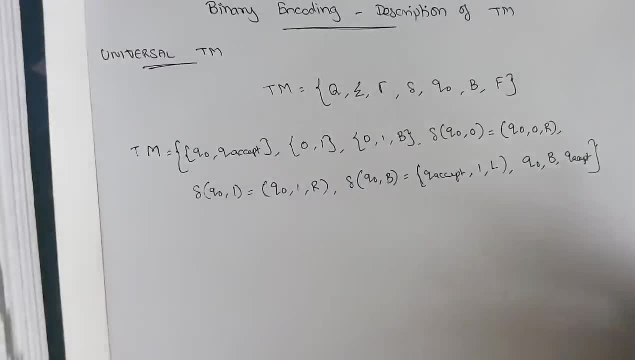 we have Qexcept as the accepting state. that is, your final state. So this is an example of a Turing machine. Now we are going to convert this to an encoded format. Encoding is a very simple one. I will just say you what it is and whenever the Turing 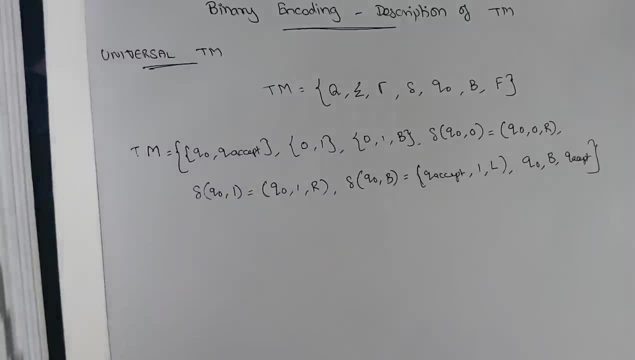 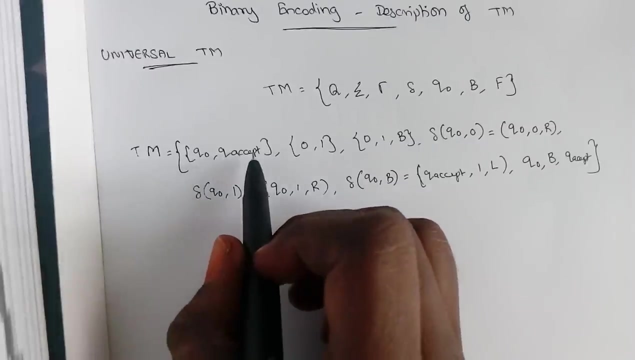 machine enters into this accepting state on some input, the universal Turing machine has to accept it. So the description here is very simple, whereas, like each and every element, is represented in terms of number of bytes. For example, when I have set of states as Q0 and Q1,, I represent Q0 with a single one. 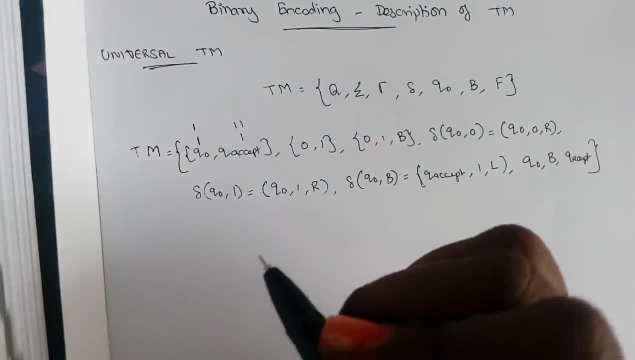 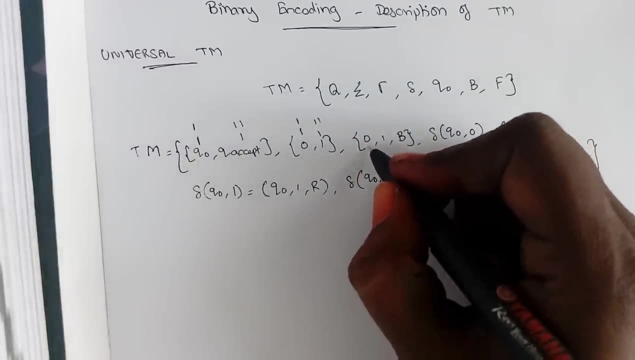 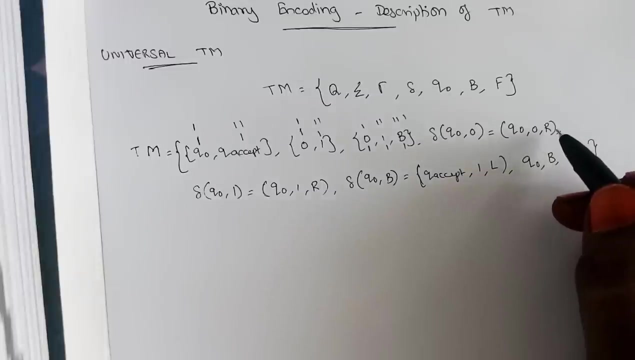 and Qexcept with two 1.. Ok, and again: 0 as a single one, 1 as two ones. So whatever element we have it over here, that is 0 as a single one, 1 as two ones and blank as three 1s, and whenever we write this transitions, so we have to focus on it. 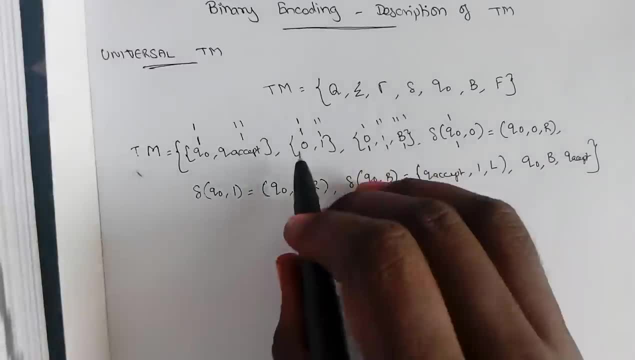 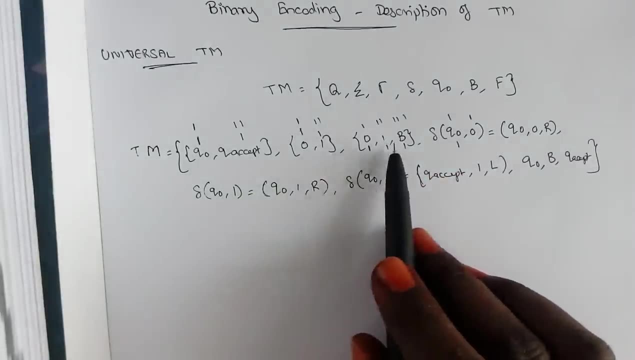 Q0. Q0 is given the value as 1,. 0- 0 is given the value as 1.. So this 0 is taken from the tape alphabet. so it is better to give the input and the tape alphabet to Q1.. alphabet, like when you have a 0 in input and 0 in tape alphabet: give the same value. that will be. 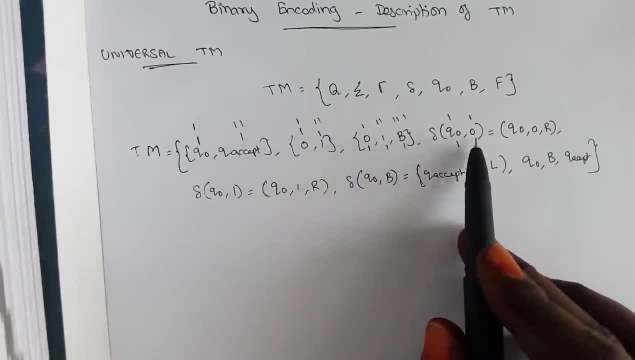 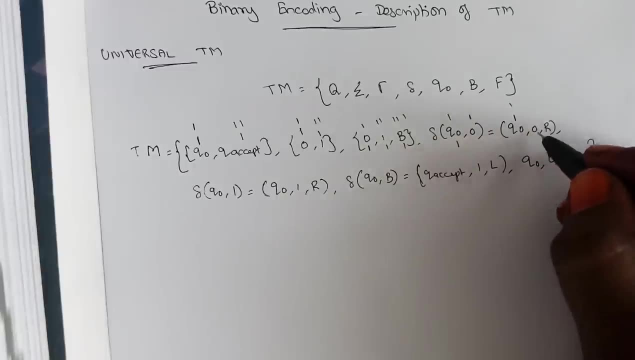 easy for you to do. okay, if you change this order you will get confused of it anyway. this 0 describes the element that is taken from the tape. and again, this q0 value is 1, 0 tape element value is 1 and for left and right side mu give a. when it is left side mu give the value as 1 and right side mu give. 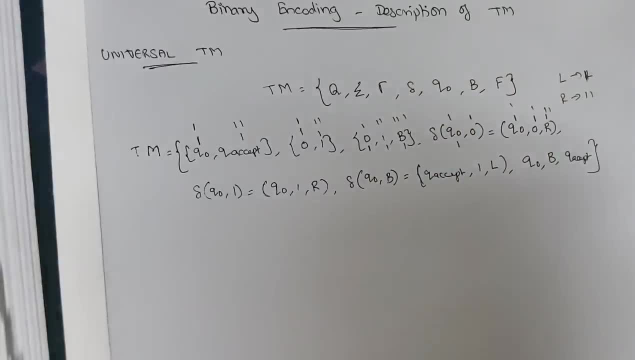 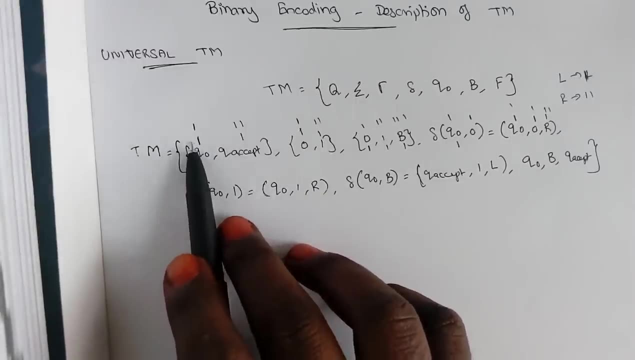 the value as 2: 1's, so it is 2: 1's. okay, so this is how it is described and, to make this difference, this 1 is your q0 and the next element is the next input. so, in order to make the description, 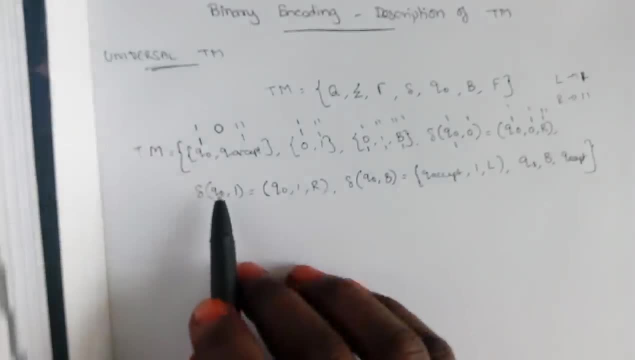 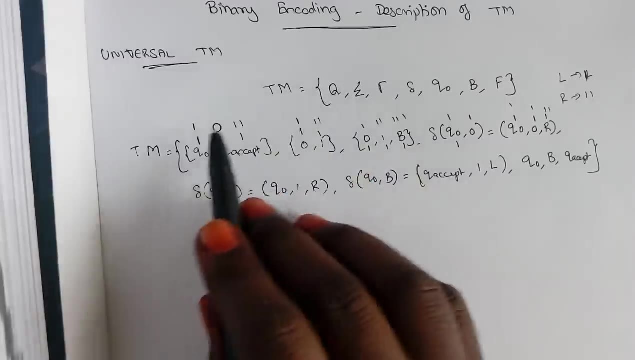 difference, you use the 0. okay, and again this 0, a single 0 represents the difference in each and every element, in a element, like when you have q, when you have 2 or 3 element, 2 or 3 states, that states are distinguished with this. 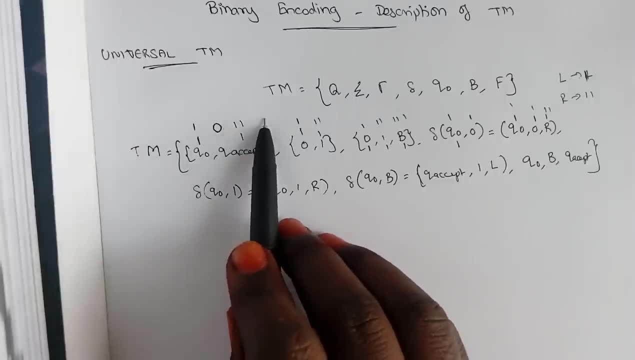 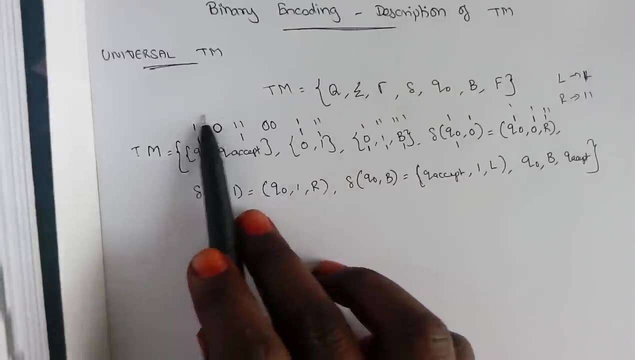 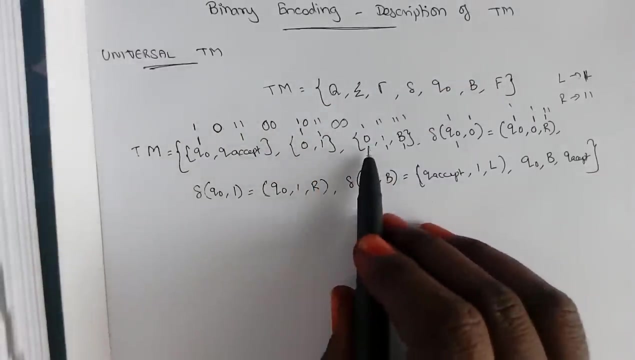 single 0 and when you differentiate this states with that of input symbol, use 2: 0's to represent it. okay, so when you have 2 0's, this is your first element, that is your set of states. and again, when you use a single 0, this is all the input symbols and 2: 0 to separate this with the tape element. so 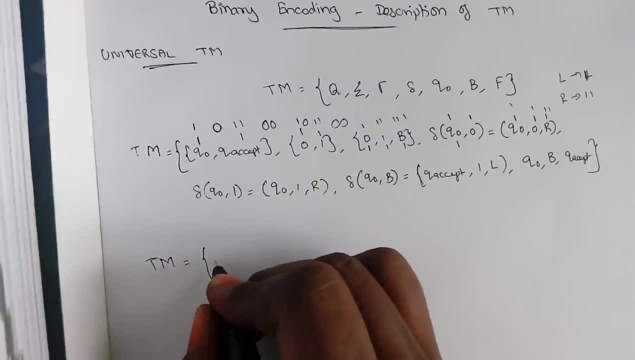 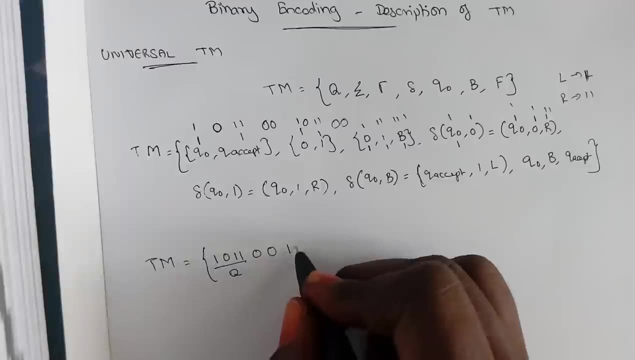 final description for a turing machine is given as 1 0 1 1. when it is double 0, this is your states and for input: 1 0 1, 1. so first input, second input, and only two inputs are there. so that is separated. so this is your. 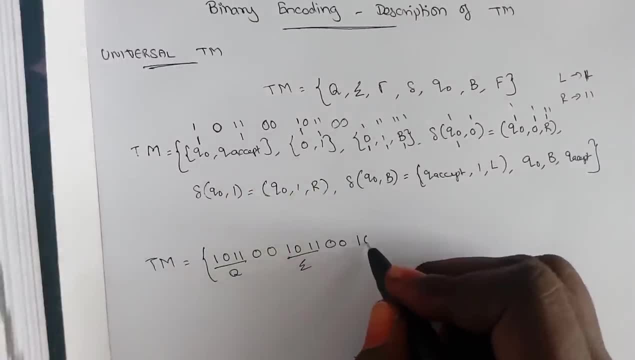 input and next one is the tape element. you have a 1 or 2, 1 or a 3- 1. okay, so this is all a bit encoded. 1, 2, 3, 3 elements are there in your tape elements and that is separated with 2- 0's. and now 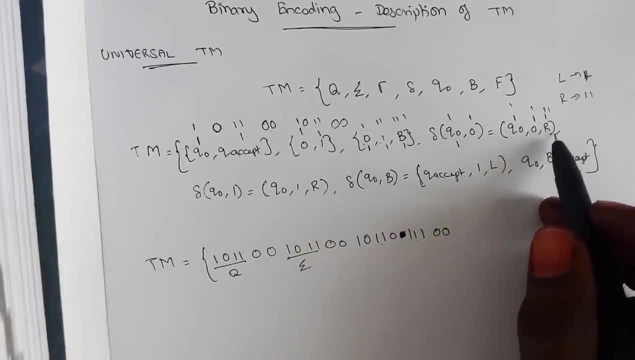 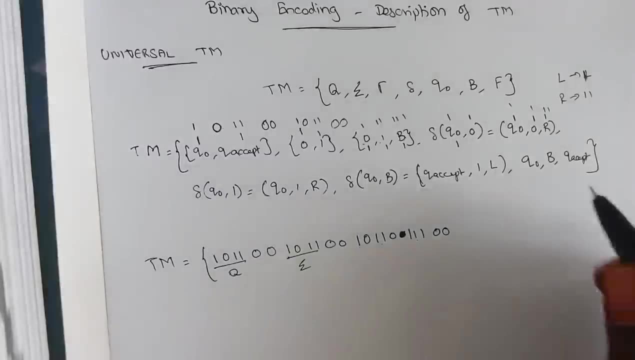 comes your transitions. so whenever you write a transition, it has 1, 2, 3, 4, 5 elements. okay, so each element over here are separated using a 0, so 1 0, 1. the transition for this is 1 0, 1 0. 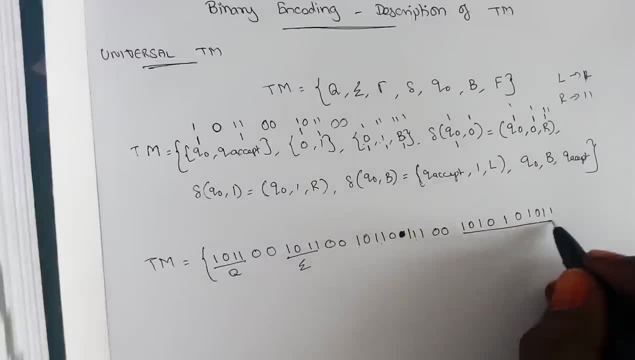 then 1, 0, 1 0, 1, 1. so this is your first transition, see 1. and this is separated with the input with the 0, and this is separated with the input 0 here. okay, and description for this is: 1, 0 is 1, 0 and the right side move we use 2: 1's to represent it. okay, so this is the 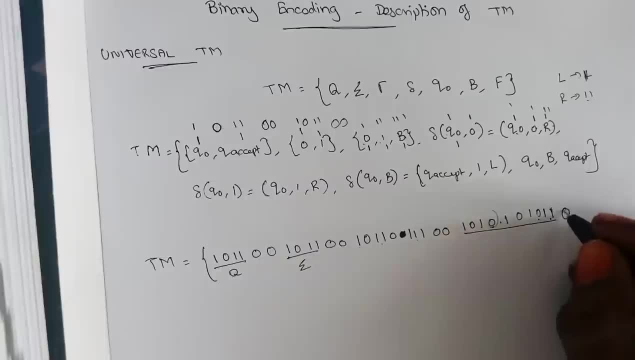 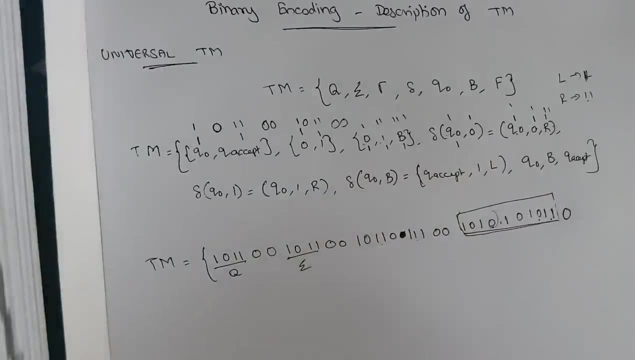 transition. okay, so this is your first transition and this is separated with a single 0 with the second transition. the reason is like this as a whole represent the transition, and transition always contains the same number of elements. okay, so when the 0's are encoded, it actually. 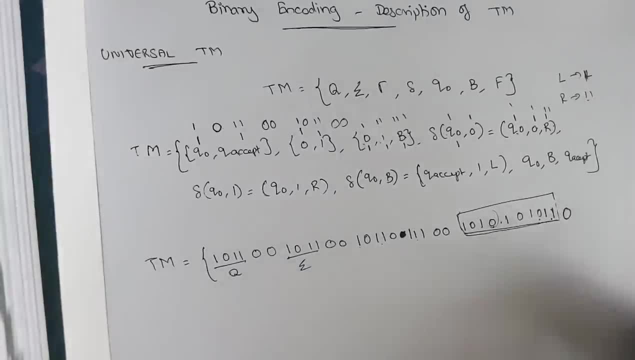 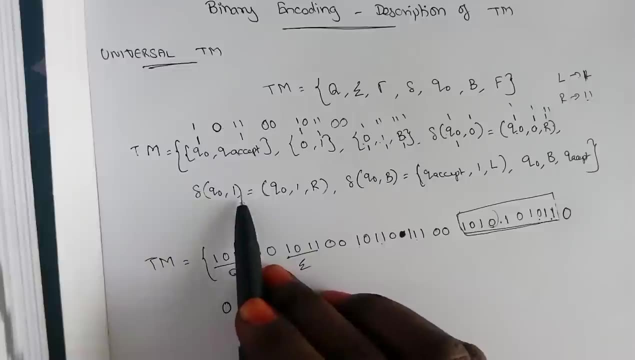 describes that this is the end of your first transition and we are going for the second transition, again for writing the second transition. q naught takes the value as single 0 and 1 takes the value as 2, 1's. okay, one, one, and it is separated with again a q naught, a single one to represent it and again. 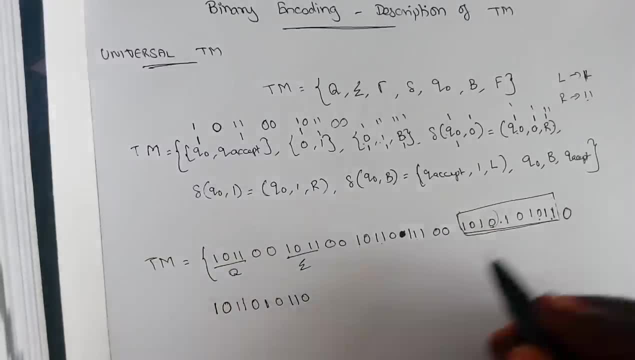 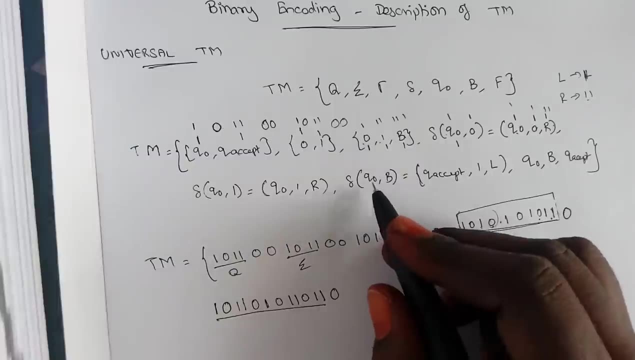 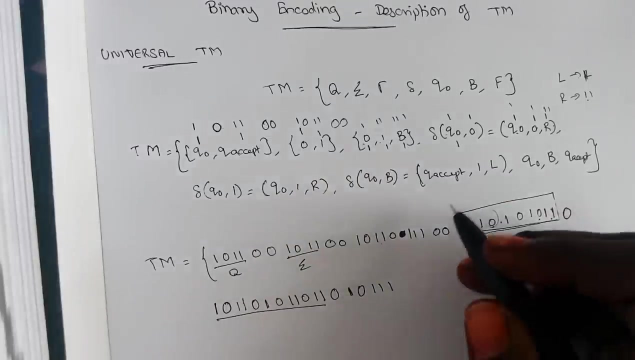 you have one, two ones to represent it and the right side move- right side move- was represented using a two ones. so this is a description for your second transition. and again, third transition: q naught takes the value of one separated by blank symbol. takes the representation of three ones separated by q. accepting state takes the value of two ones separated by this. 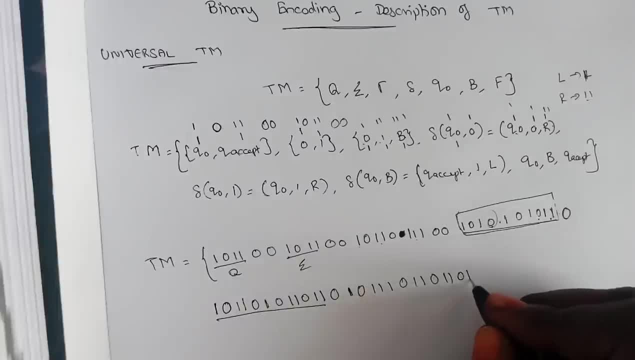 one. one takes the value of two ones, and left side move takes one value. so this is your next transition. so we have three transitions as a whole. that is described over here. so with this the transition ends. i use two zeros to represent it. and next one is your starting state: starting. 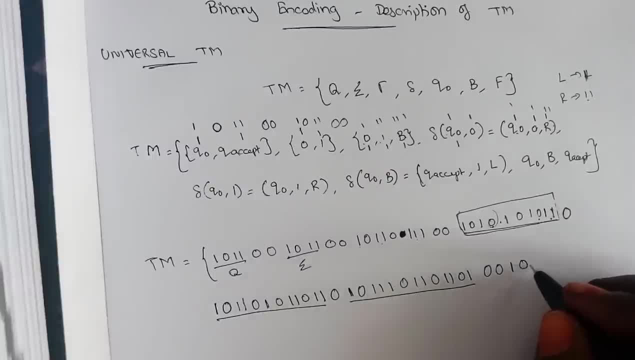 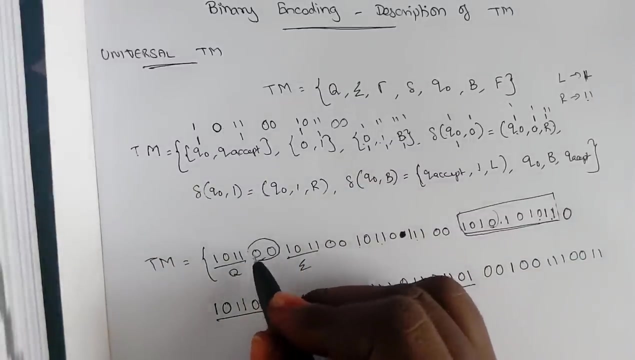 state is q naught, so that is your one and that is separated by this blank representation. we use three ones to represent this blank representation and finally, we have a q accepting states, so q accepting state is just represented using two ones. okay, so when you have two zeros, this is a delimiter for each and. 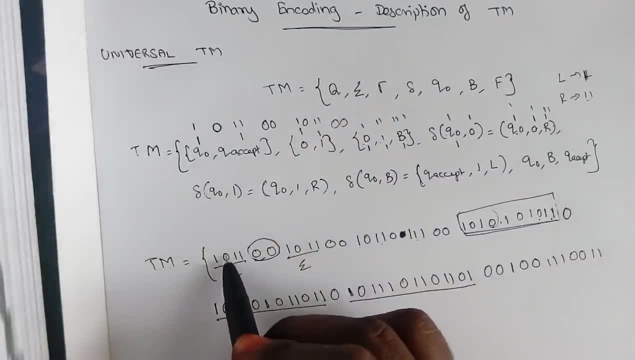 every element of a turing machine. and when you have a single zero, it is a delimiter to represents the finite set of elements inside a single place. okay, when it is state for finite set of states, we use a single zero for it. okay. so this is your del function and again this one. 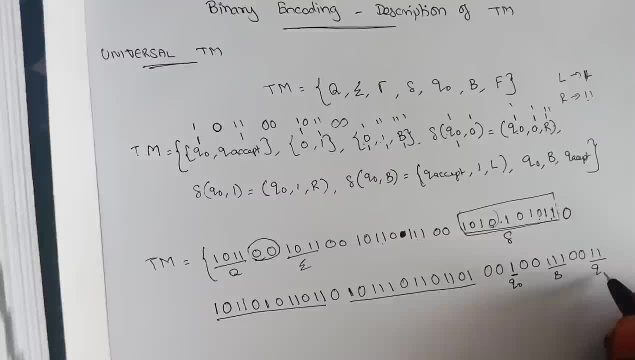 represents this q naught, and this is your blank and this is your q except. so this is a description, binary encoded, of a turing machine, and usually we use a representation of turing machine as m comma w. okay, so when you run a turing machine, we have a machine description along with the input symbol. so we have to describe. 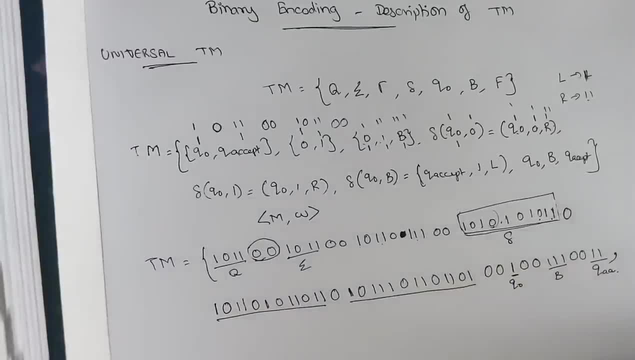 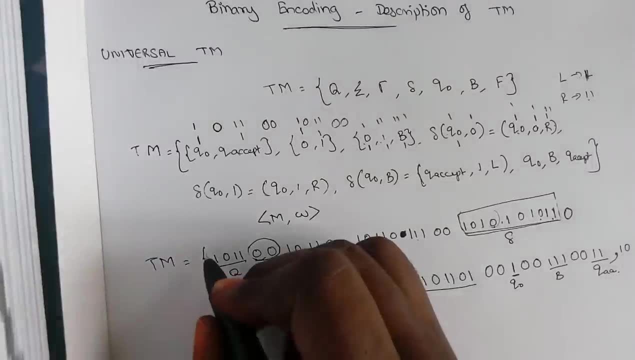 both the input and the machine. so we use a comma as a separator over here and we can write whatever is the input, my, if my input is one zero, i use it. a representation like this: so this is your description of a turing machine. i give it like this. okay, so this is called a binary.